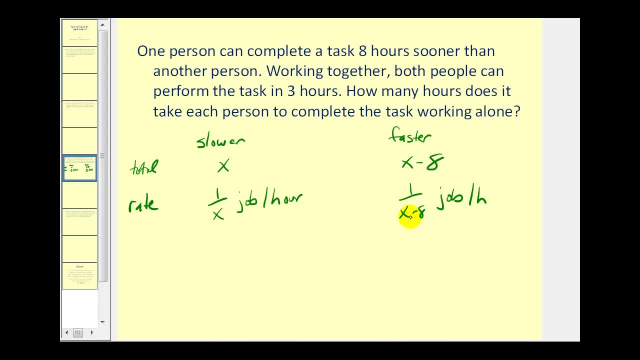 complete a job, the reciprocal would be the rate per hour for that job. In the problem it states that working together they can complete the task in three hours, which means their combined rate would be one-third of the job per hour. So with all this information we can get an equation where 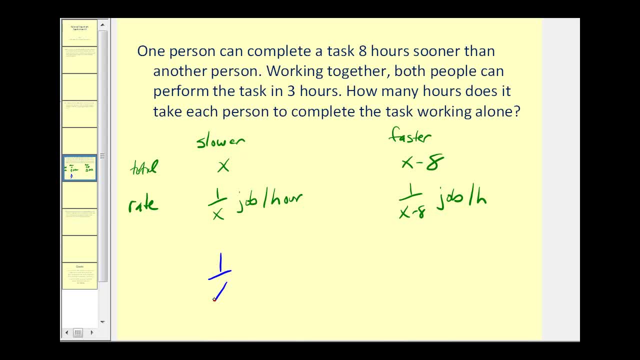 the rate of the slower person plus the rate of the faster person must equal the total rate which, again, if it takes three hours, would be one-third of the job per hour. So this is the equation that we have to set up and solve in order to determine how long it will take each person working alone. 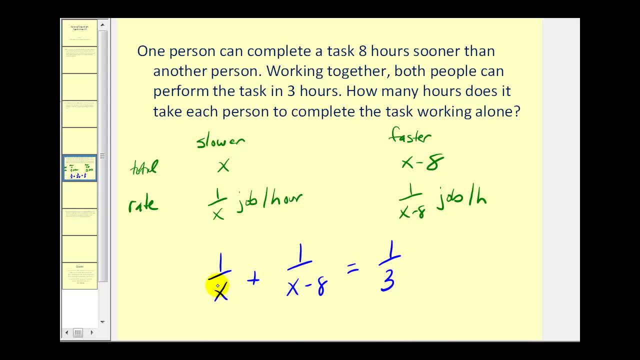 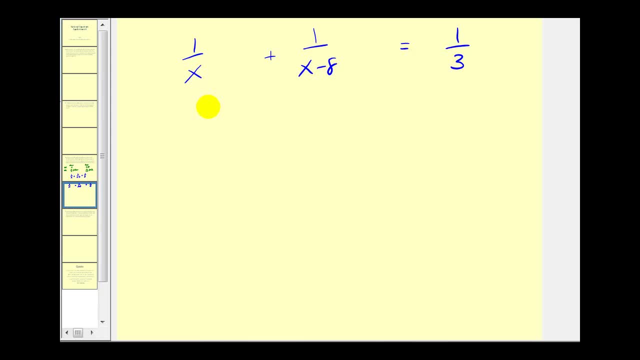 Let's take this over to the next screen and solve this. So we have a rational equation here. We'll multiply both sides of the equation by the LCD or least common denominator, which would be the product of all three denominators. So we have to multiply each of these by 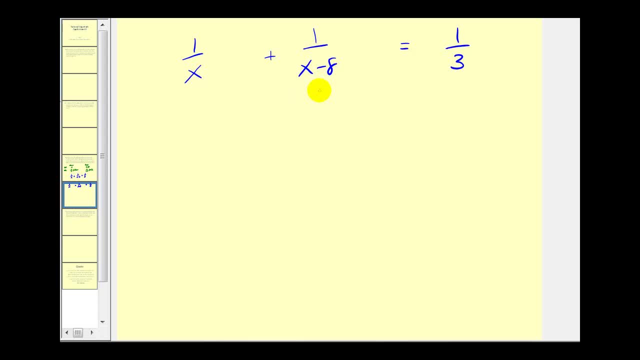 three times x times x minus eight. Let's go ahead and set this up. So notice, we're not obtaining the common denominator. we're multiplying each term by the LCD over one. Let's go ahead and simplify. Notice, here the x's simplify out. 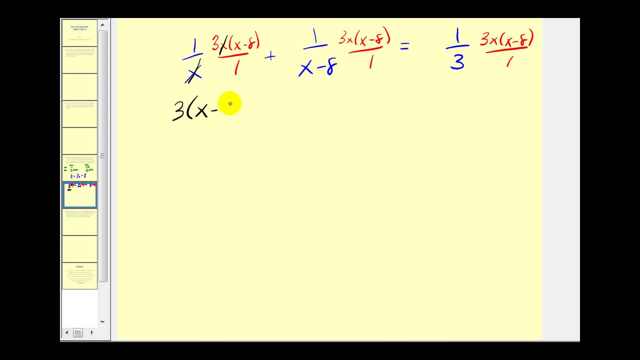 We're left with three times x minus eight, plus- here the x minus eight. simplify out. We're left with three x equals- Here the three simplifies out: We're left with x times x minus eight. Let's go ahead and clear the parentheses, So we'll distribute the three. 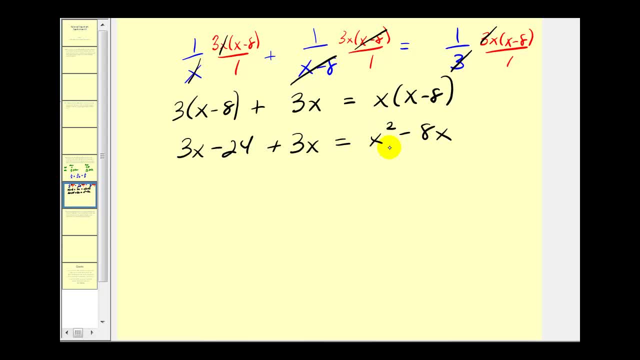 Distribute the x. Notice we have a quadratic equation. Let's go ahead and clean this up. Set it equal to zero and see if it factors. So here we have like terms. So it would be six x minus twenty-four. Now let's go ahead and move these terms to the other side. We'll add twenty-four to both sides. 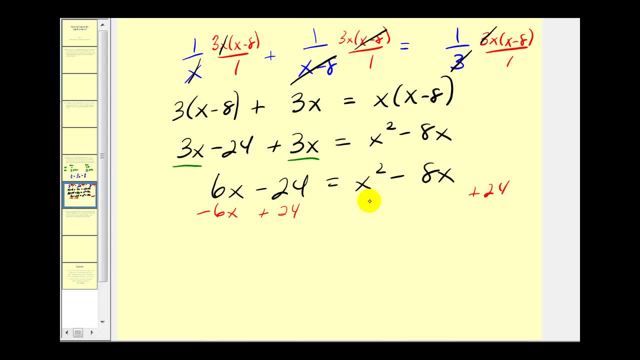 and also subtract six x, So we have zero equals x squared minus fourteen. x plus twenty-four Looks like this will factor the factors of twenty-four that add to negative fourteen, Negative twelve and negative two, So it looks like x equals twelve or x equals. 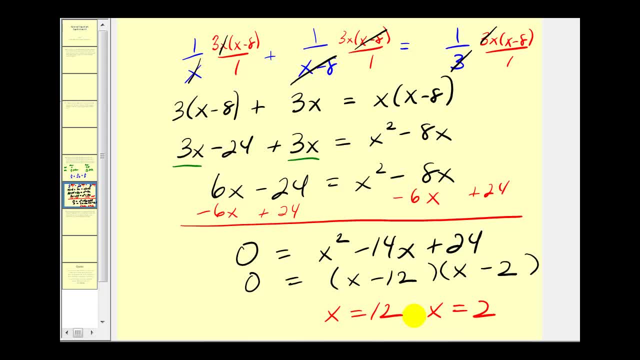 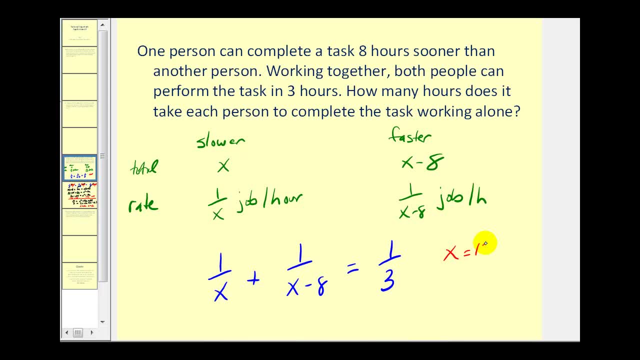 two. Let's go ahead and go back to the original problem and check these solutions Again. the possibilities were x equals twelve and x equals two. Let's take a look at x equals two first. Remember the question wants us to determine how long it takes each person. 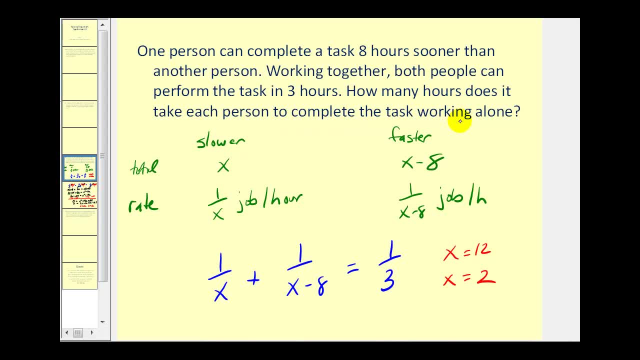 to complete the task alone, And that would be x and x minus eight. The problem with x equals two is that we can't have a time that would be negative. Two minus eight is negative six. That doesn't make sense. So x equals two is an extraneous solution. Let's check twelve. 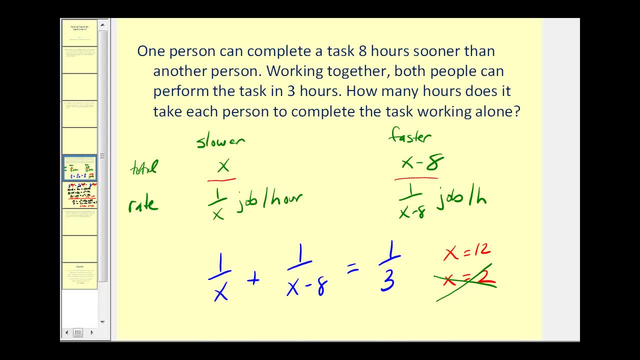 If it takes a slower person twelve hours, well, twelve minus eight, that would be four hours for the faster person. So those are the two answers we're looking for. The slower person would take twelve hours working alone and the faster person would take four hours working alone. Let's take a look at 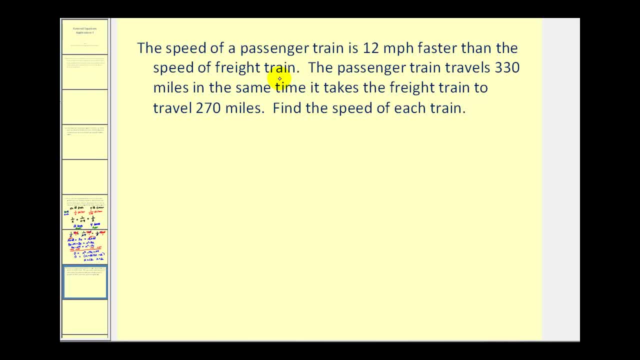 another problem. The speed of a passenger train is twelve miles per hour faster than the speed of a freight train. The passenger train travels three hundred thirty miles. in the same time, it takes the freight train to travel two hundred seventy miles. Find the speed of each train Okay. so the first thing we have to remember is that 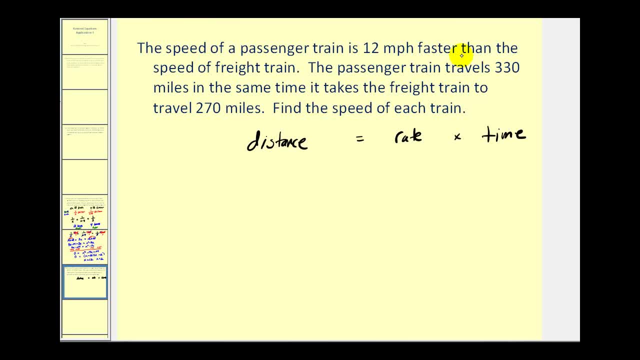 distance equals rate, times, time. So the first thing we're going to do is just record all the information that's given in this question in a table. So we have distance, rate and time, And we also have a passenger train and a freight train. 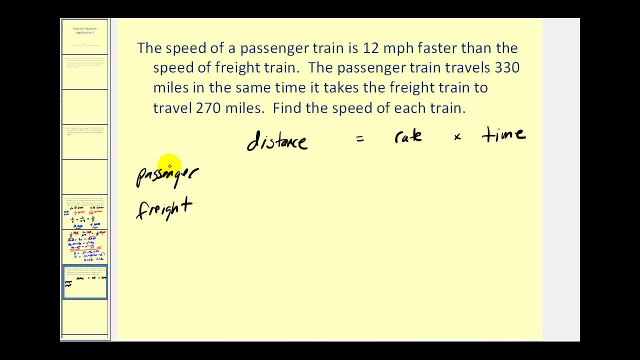 So it says the speed of the passenger train is twelve miles per hour faster than the speed of the freight train. So the passenger train is twelve miles per hour faster. So if we let the rate of the freight train equal r, then the passenger train 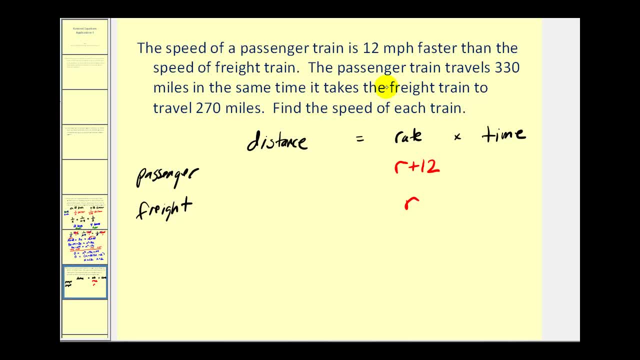 would be going r plus twelve miles per hour. Next, the passenger train travels three hundred thirty miles. in the same time, it takes the freight train to travel two hundred seventy miles. There's a very important detail in here. It says that they travel these two distances in the same time. 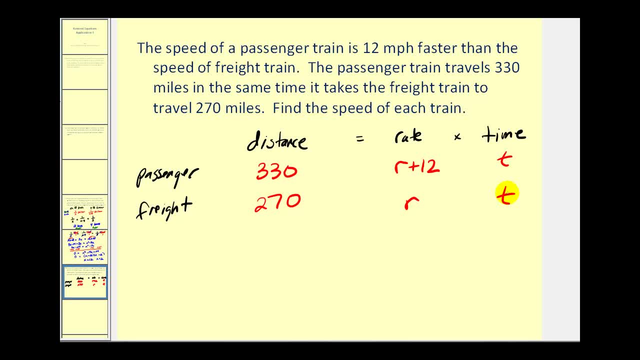 So whatever t is, it's the same. So if I use a t here, I can use a t here as well. Again, we know that distance equals rate times time. If I was to solve this equation for t, we would have: the time must equal the distance. 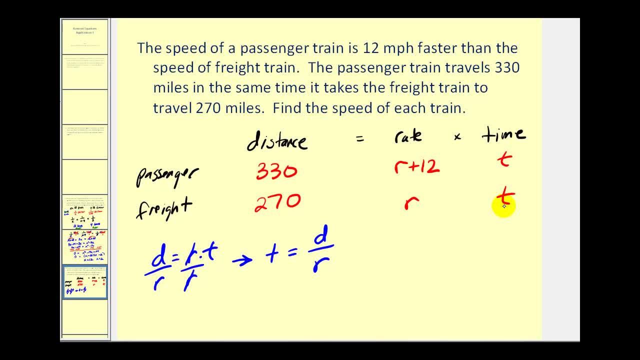 divided by the rate. The reason this is so important is if these two times are the same, then the distance divided by the rates must equal each other. Let me say that again: If these two times are the same, then it must be true that the distance divided by the rate must also be the. 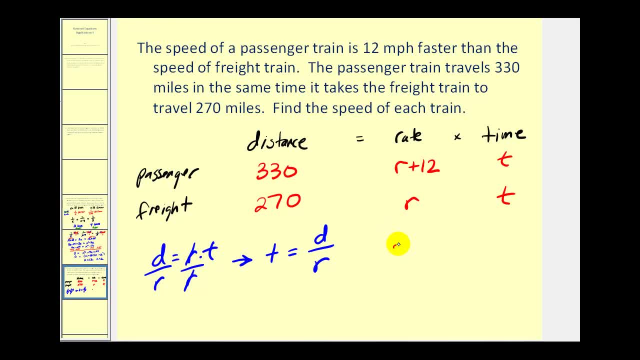 same. So what we can do is write an equation where we have: the distance divided by the rate for the passenger train must equal the distance divided by the rate for the freight train. So this is the equation that we have to set up and solve. 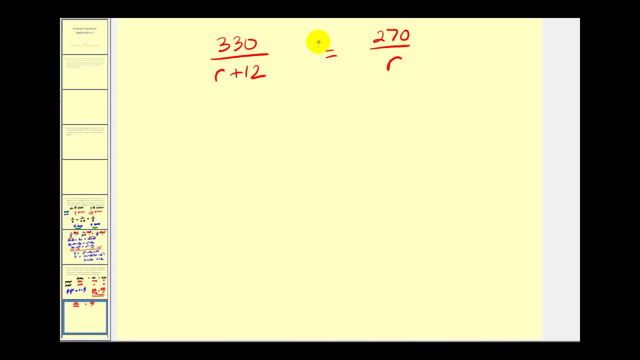 Again. let's take this over to the next screen. This is a proportion, so we could cross, multiply, but I'll go ahead and keep it consistent and multiply every term by what would be the LCD, And in this case the least common denominator would be r times r plus twelve. 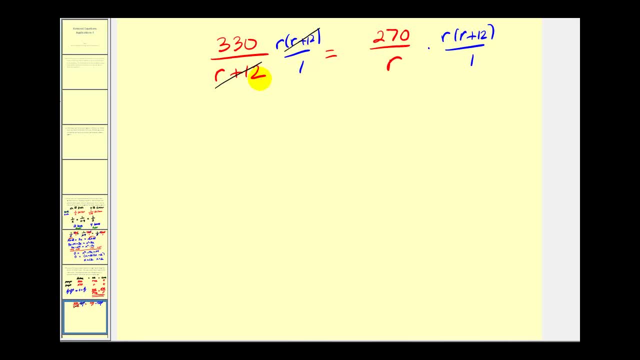 So when we simplify here the r plus twelve simplify out, we're left with three hundred thirty ohms. So r must equal. here the factor of r simplifies out, we're left with two hundred seventy times r plus twelve. Let's go ahead and solve for r. 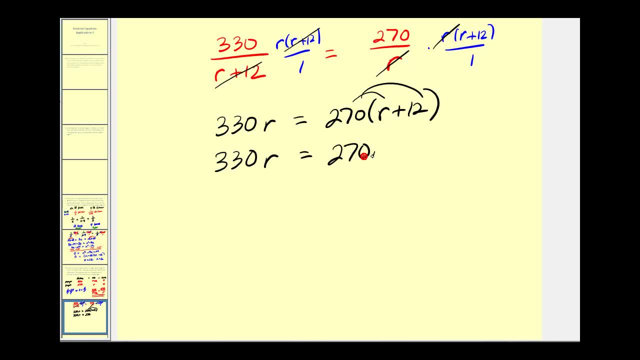 Let's go ahead and clear the parentheses here. We'd have two hundred seventy r plus two hundred seventy times twelve is three thousand two hundred forty. Let's go ahead and subtract two hundred seventy r on both sides. This would give us sixty r equals. 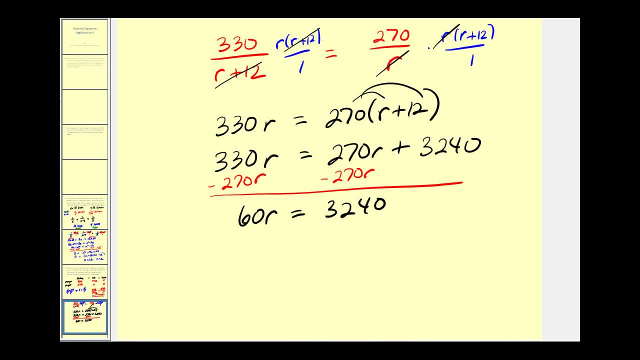 three thousand two hundred forty Divide both sides by sixty, So r is equal to fifty-four. I believe it was miles per hour. Let's go back and make sure we answer the question now. And we did find that r was equal to fifty-four miles per hour.